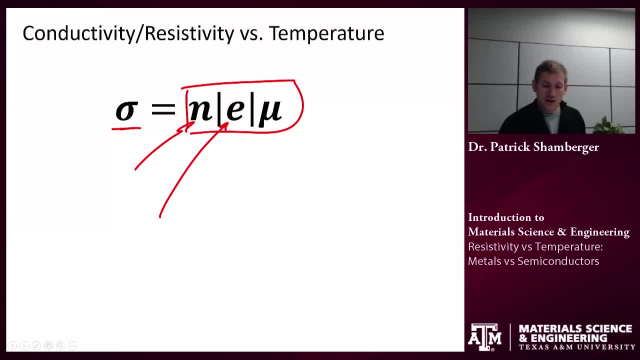 in the system. So how many particles do I have moving around? E is the charge. So if this is just an electron, then we have a single electronic charge. If it's an ion, it could be a multiple of the electronic charge, And mu is the mobility. How easily do these carriers 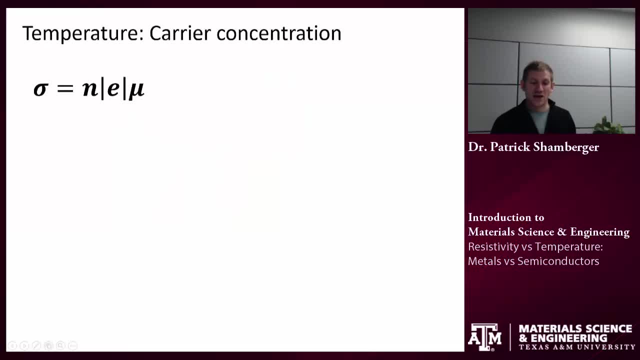 move around. So let's think about how conductivity affects conductivity and resistivity. We want to think about how does temperature affect each of these terms differently. First we're going to think about n: How does temperature affect the number of carriers in a system? So when 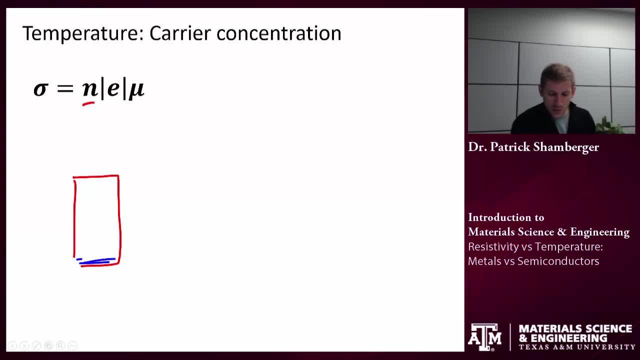 we drew occupied bands before. we would always occupy them from the lowermost energy up to the point where we ran out of electrons, And we call that highest occupied energy Fermi level. Now, this is a nice picture, But it actually is a little bit more complicated than that, Because at any given finite temperature, 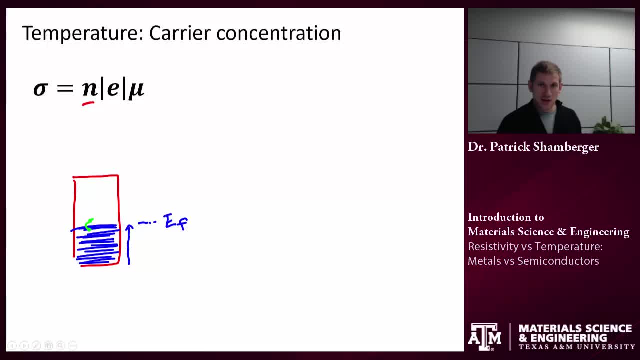 we're exciting some of these electrons up to higher energy levels, And the amount that we excite up is going to be related to the temperature in the system. So if I have something that's exactly at zero degrees Kelvin, perfect zero, then I will fill up to the Fermi level. 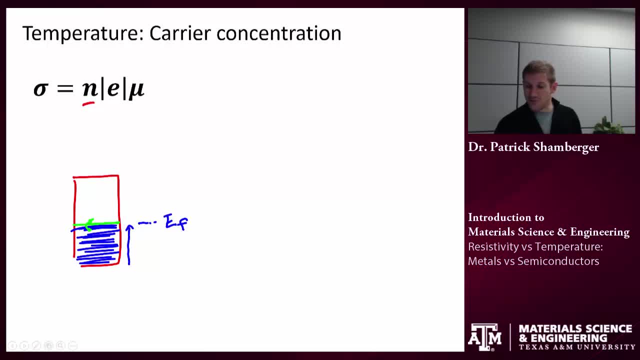 and stop And I will have no occupied energy levels above that And then any temperature greater than 0K. I'm going to have some sort of distribution And it'll look something like this. So this is a probability distribution of occupation of these different energy levels. 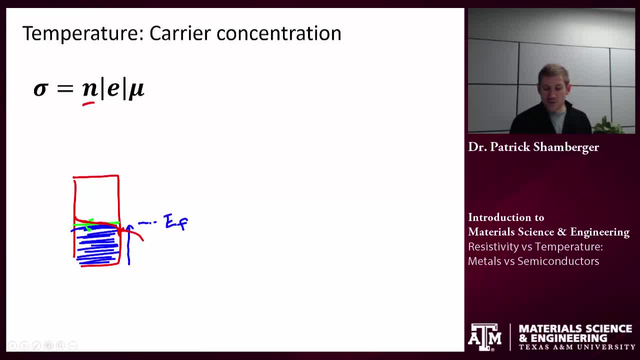 So at some energy a little bit below the Fermi level, maybe I have a 95% chance of occupying it. At some energy a little bit above, maybe I have a 5% chance of occupying it. The larger the temperature is, the more I'm going to have some distribution to that energy. that's. 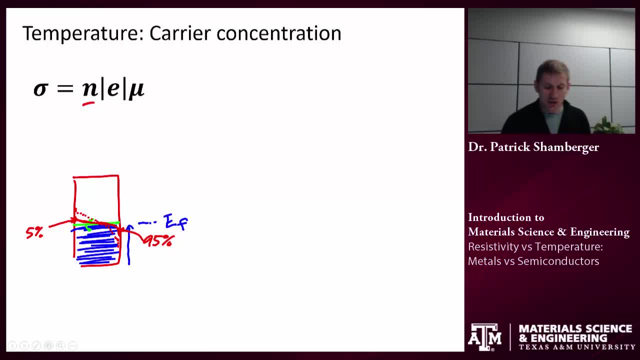 the more smeared out this distribution becomes. So this is called the Fermi-Dirac distribution And basically it's talking about what are the energy levels that the electrons will actually occupy at some finite temperature. The important thing to remember here is that the higher the temperature is, 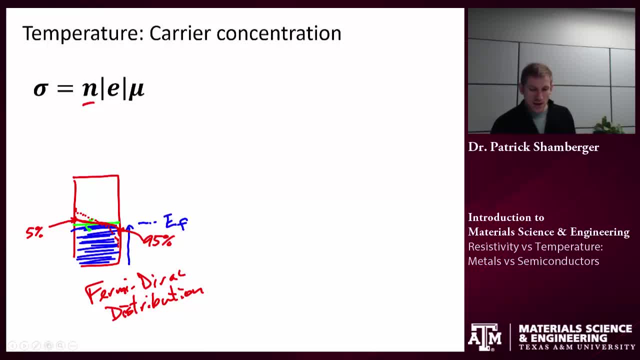 the more smeared out that occupancy will be. Now in metals this does not actually matter that much because we already have a large number of carriers at that Fermi level. So if I increase the temperature a little bit it's not increasing the number of carriers all that much. 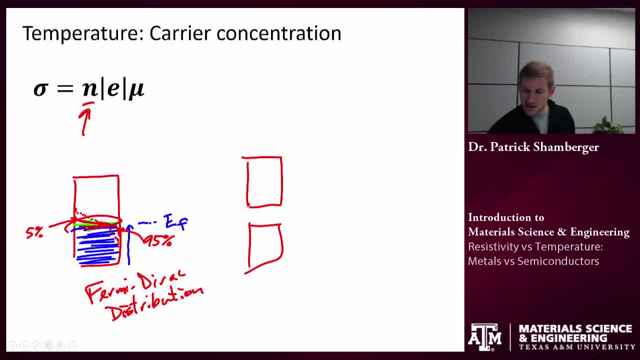 That's different from the semiconductor case, because in this case my Fermi level will be somewhere in here, but at zero kelvin. I would have no electrons excited up to the conduction band from the valence band At any temperature above that, though. 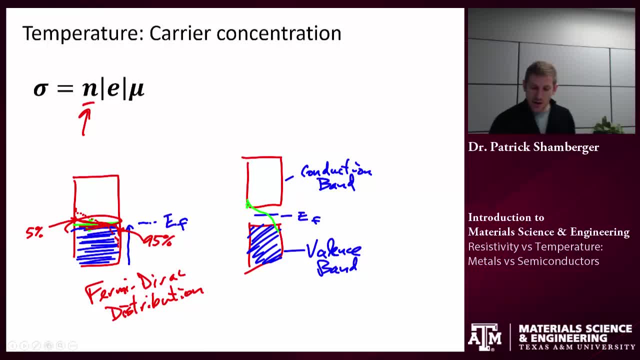 I'm going to have some small number of electrons that gets excited up, And the greater the temperature is, the greater the number of electrons that get excited up. So that's the number of free carriers I'm going to have. Now, remember, our semiconductors tend to be carrier starved. 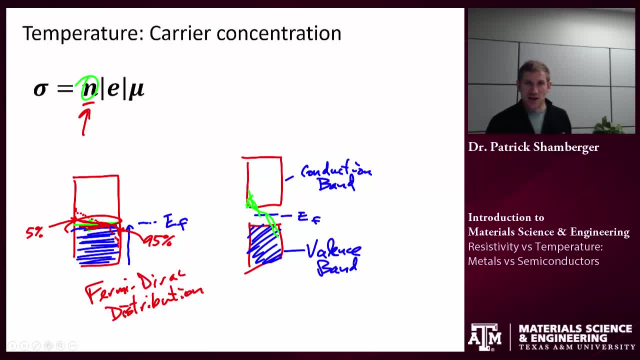 So increasing that number of free carriers has a very large impact on semiconductors. as opposed to the metal case, So that was N. The charge is temperature independent, so that's not going to change. But next we need to focus on the mobility. 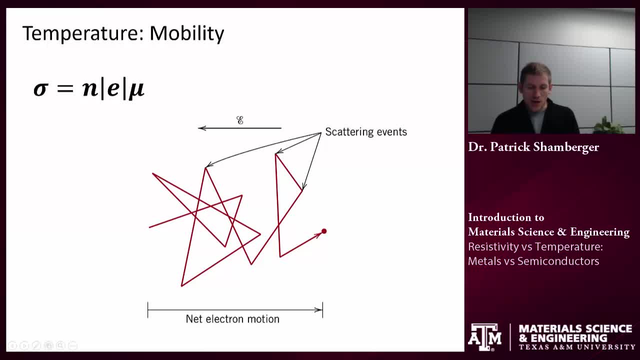 Mobility. we need to think about these free carriers moving around, And when they hit some sort of defect, something that's a little bit out of place, they tend to scatter. So an electron does not flow smoothly from a high energy level to a low energy level. 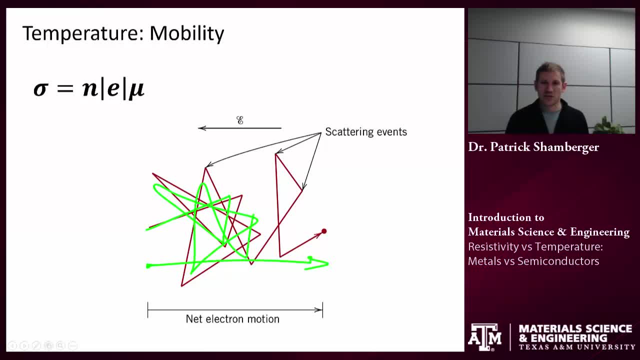 It is going to scatter repeatedly. So we have this picture of electron path, and the path is actually a bunch of small distances that get traveled before it hits that next scattering site. So as the temperature increases, atoms tend to vibrate more and more. 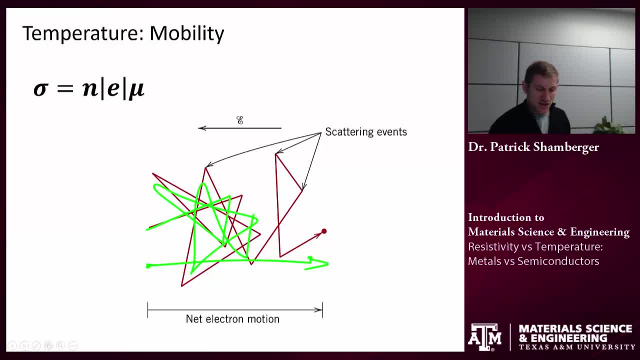 And so I tend to have more scattering events. So as temperature increases, the mobility decreases, It's harder for electrons to move around in the system. This is going to affect both metals and semiconductors, Although- remember- semiconductors are number of carriers.